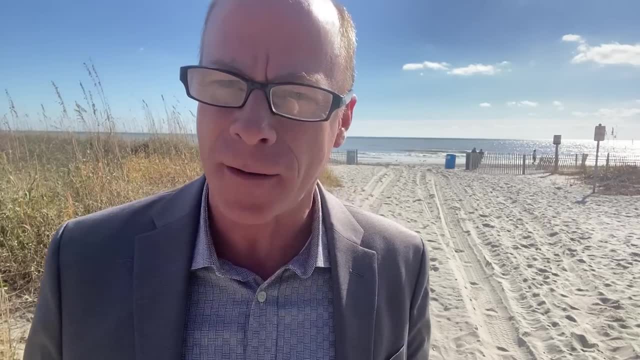 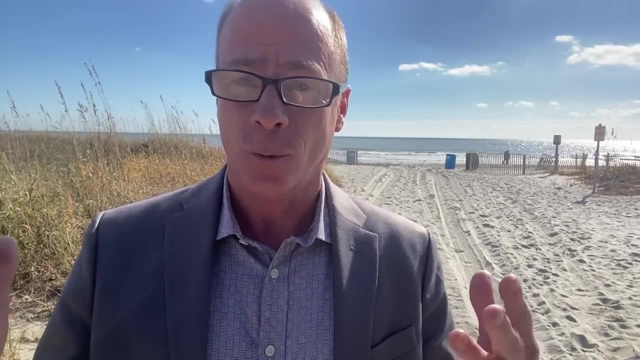 us about for the last three years? Where's all those 50% off deals And where's all the affordable houses? What's really going on here, guys? The truth, this runaway inflation is still affecting us every single day and we're not headed in the right direction, And you know how. 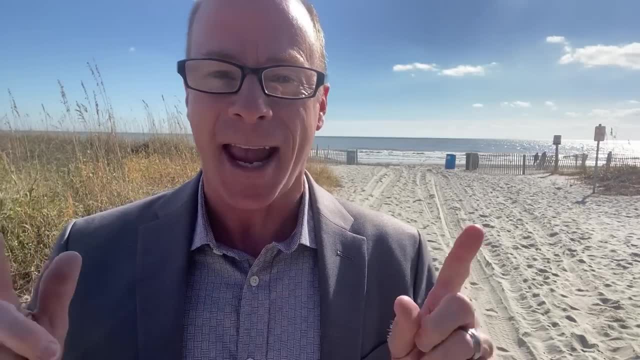 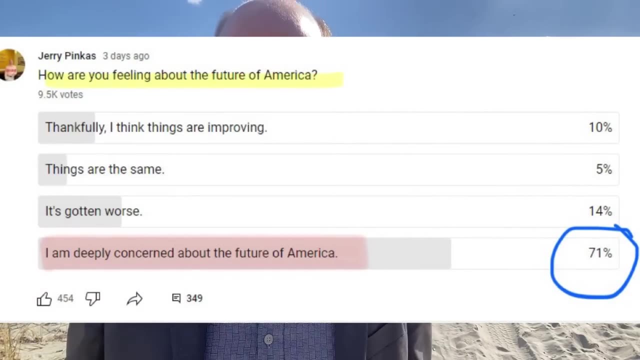 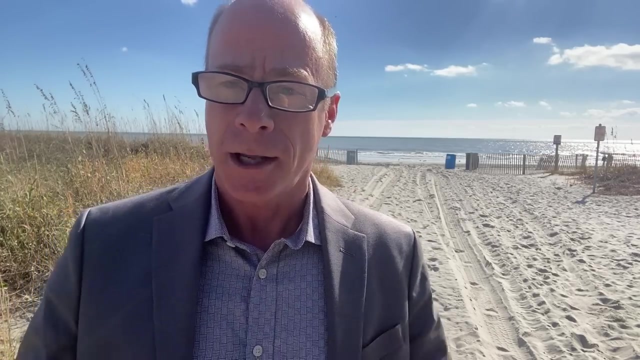 I know this, You guys told me. so I did a poll with 8,800 people here on this channel and 70% of you said you're deeply concerned about the future of America. So what will happen with housing, real estate and the economy in 2024?? Now you've got to look at the broader economic 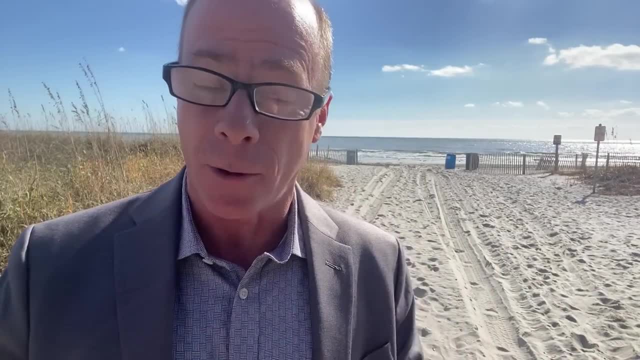 trends, the stuff that no one else is looking at, to figure out what's really going on here. And this is why I'm doing this: It's to educate the public. So if this is your first time here, I just want to say: 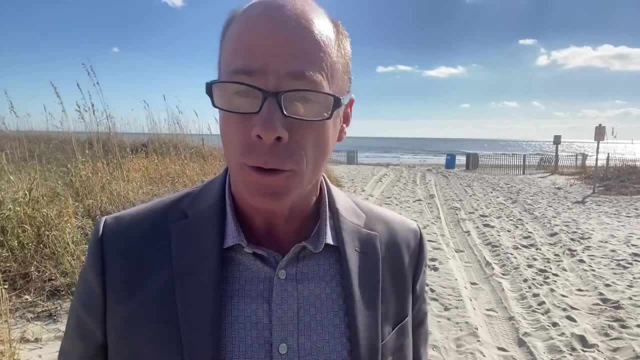 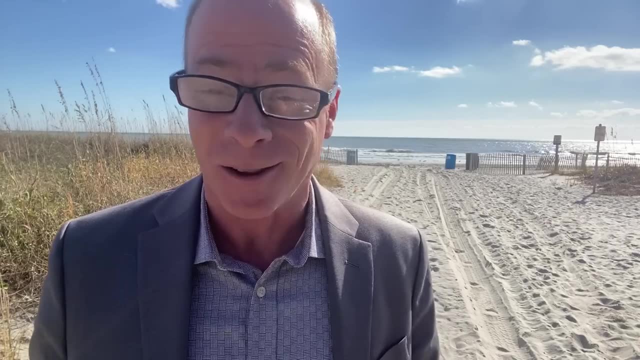 welcome aboard. This is the Real Estate Channel. It's all about helping you to avoid the pitfalls that are costly, So give me a thumbs up if you're good with that. Now, look, we've all been lied to, and I'm not talking about Santa Claus, werewolves or unicorns. I want to give you the 10 things that. 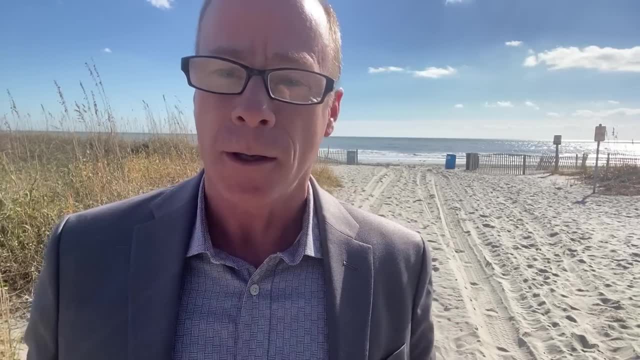 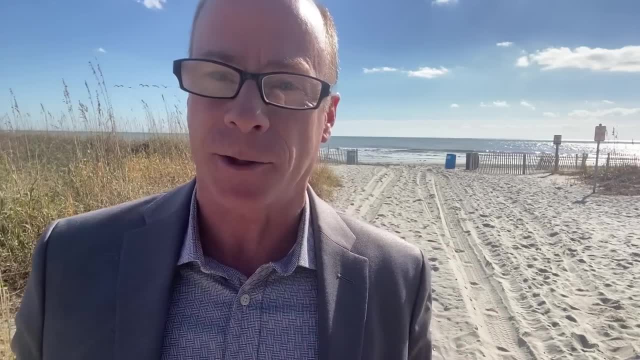 Federal Reserve will cut interest rates in 2024.. The Federal Reserve will cut interest rates in 2024.. And they're being very clear about this. They say three times: they're going to cut the rates by the end of the year. Now, when they cut interest, this is going to act as a stimulus to the economy. So keep in mind that their goal is to get inflation down to 2%. Now, we've recently not seen inflation anywhere near that low. So the question I have for you is: what have you bought this year that went up only 2%? Go ahead, put it in the comments. Now, this is the part that's: huge guys. The 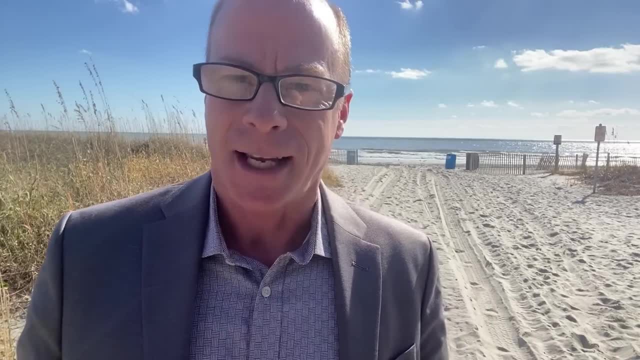 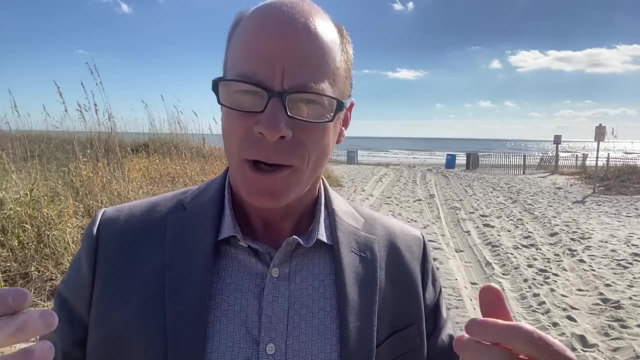 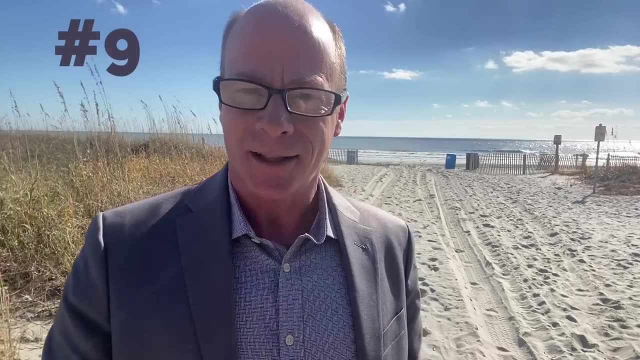 Fed is going to be at 2%, but their projections are saying that they're going to get to this goal in the year 2026, which is many years away. So do you know what happens between then and now when you stimulate the economy? Right, So, which leads us to number nine unemployment Now. 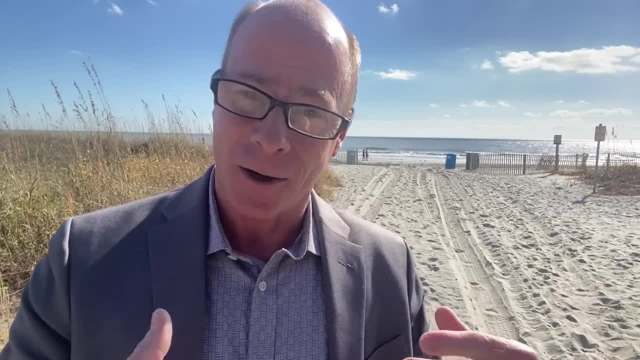 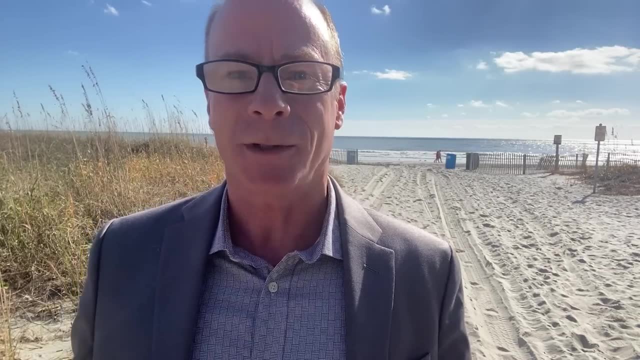 in terms of economy. just put this in perspective: In the year 1980, unemployment was at 7.8%, But during the depression in 1933, unemployment was at 25%, And the Federal Reserve is projecting unemployment rates to be at 3.8%. 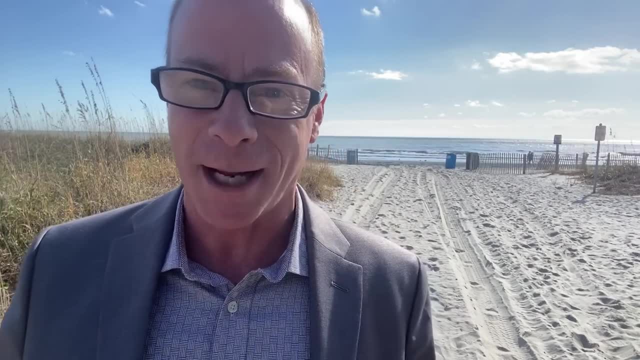 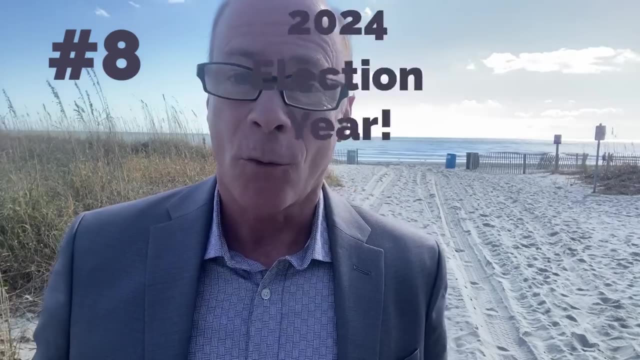 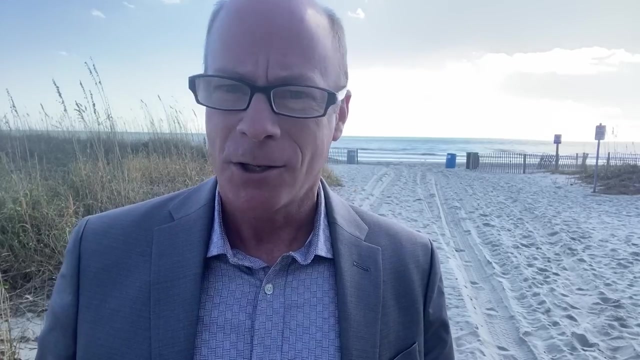 this year and go up to 4.1% in the next three years in a row. With those kind of numbers, that's some low unemployment. Number eight: 2024 is an election year. So what's motivating the Federal Reserve to cut interest rates? Because usually you do this when the economy is suffering. 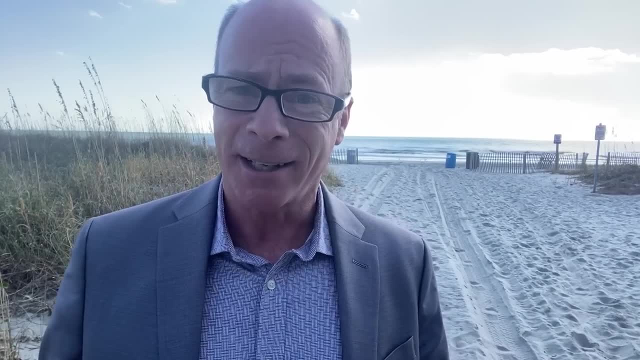 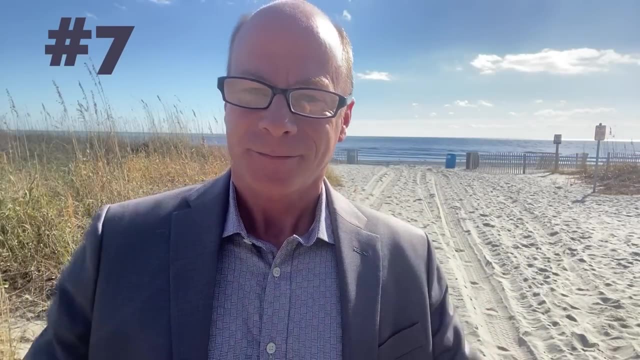 and it's doing really bad. Yet they keep telling us that we're not in a recession. So let me know what your thoughts are. Go ahead, put it in the comments, Number seven. So what is the motivation to cut interest rates? Now the government and the Federal Reserve is telling us. 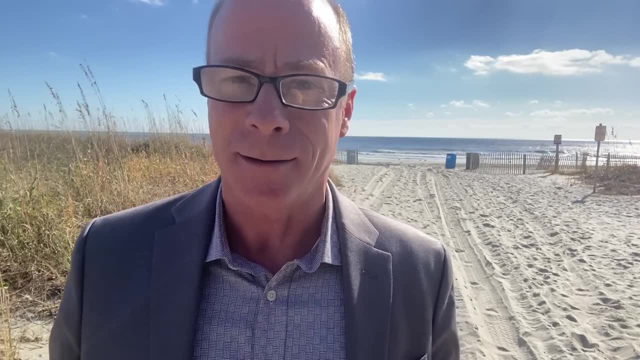 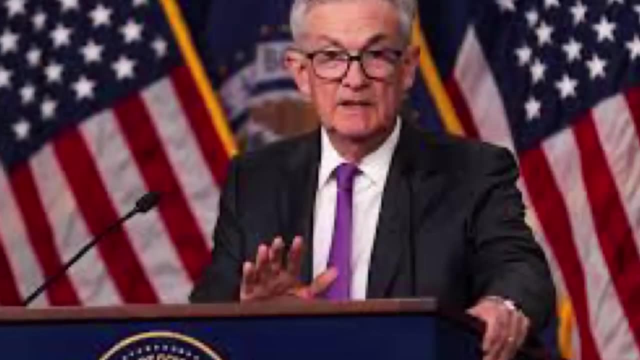 that consumers are strong, the economy is doing great and unemployment is low And the government reports are just looking fantastic. Yet Jerome Powell tells us, and I'm going to quote this: core inflation has been sticky, but there's been real progress in the non-housing sectors. 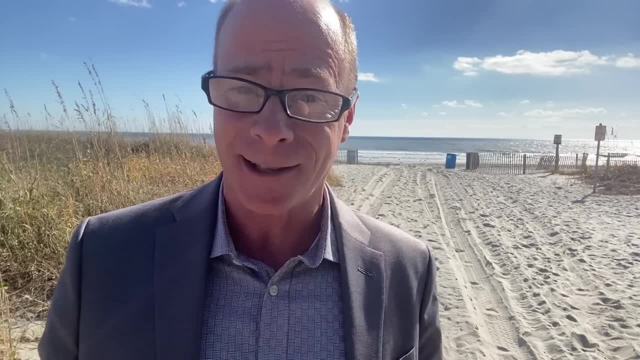 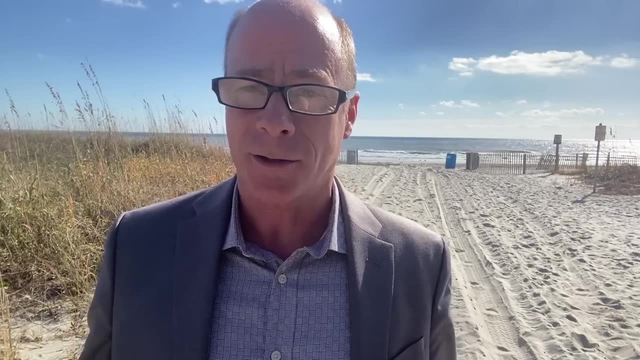 Non-housing. So does this mean that the housing service sector will continue to see price increases? I mean just read between the lines. Is that code for the US housing inventory? The number of homes on the market will still be at record lows And some buyers who have taken a breather and are sitting on the sidelines, but when these interest rates drop, we could see an either feeding frenzy or higher prices again. Well, if that's your guess, then just remember this: Households were formed between 2012 and 2022. Yet, at the very same time, 11.9 million housing. 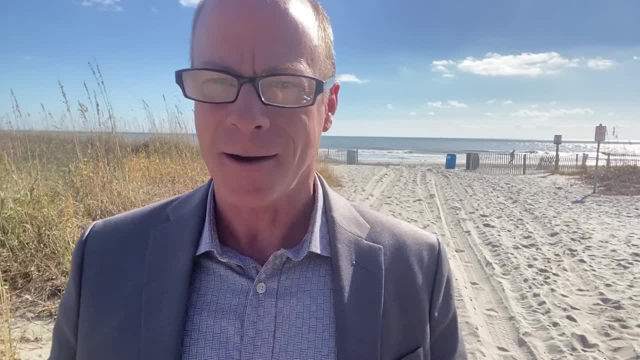 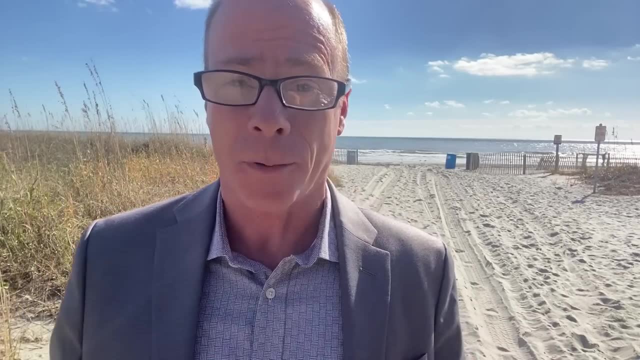 units were completed. Can you see what's happening here? We're short big time. So many of you have written me, and you've told me that it's not just the home prices, but it's the interest rates, along with affordability, that's keeping you out. So now you must keep a few things in mind if you're 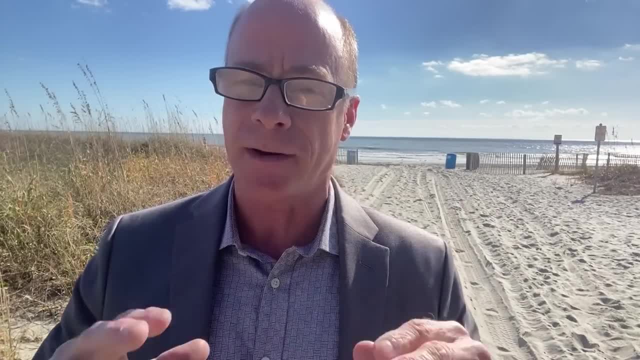 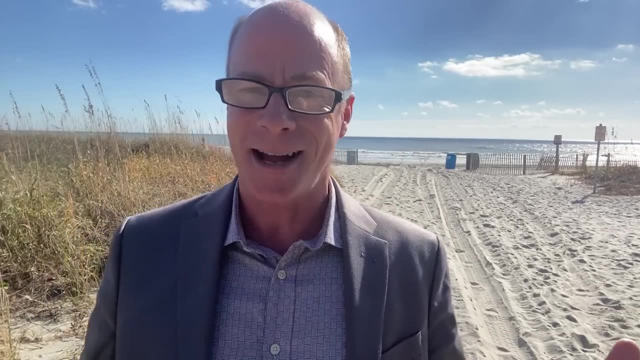 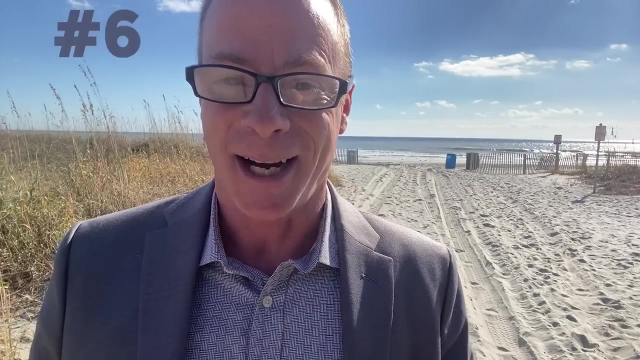 looking to buy into the future Now, over the next few years, you must have a long-term plan. We'll go into that in a few minutes. But even if you hit the lottery, that does not mean that you can buy your dream home. But at the very same time, number six we have all been lied to Look on. 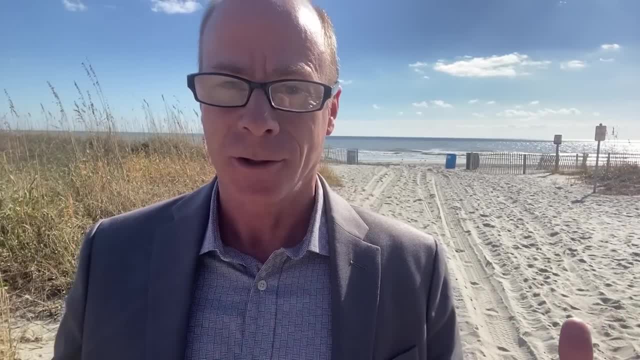 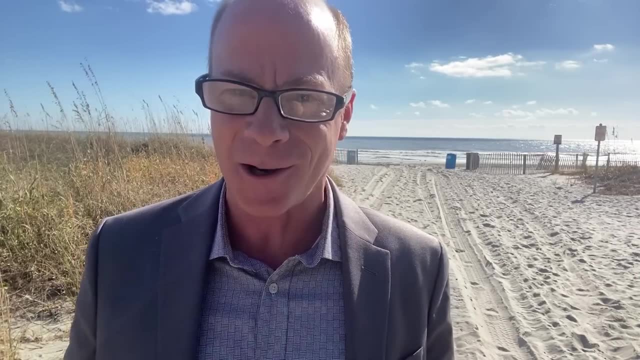 paper. you and me, we're living through the golden age, But the government reports are looking just fantastic. There's prosperity, there's wealth, And have you seen the number of fancy cars driving around? So why is this happening? Well, the government reports are looking just fantastic. 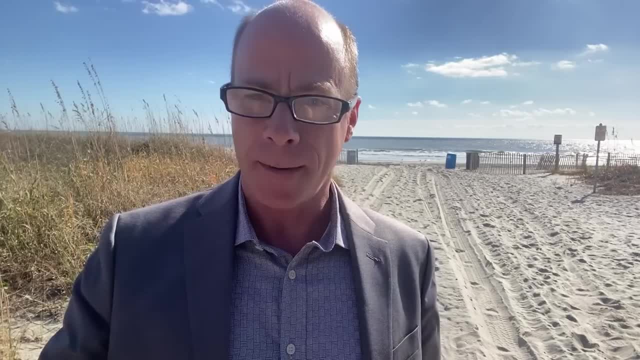 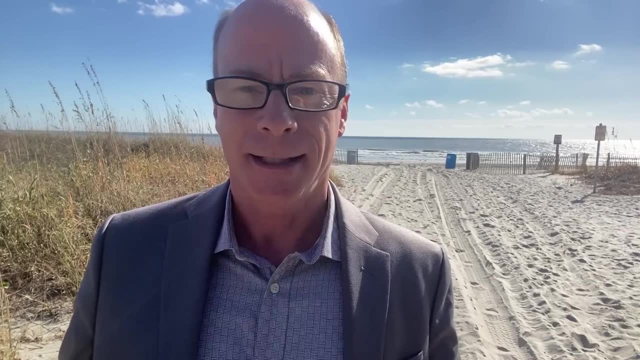 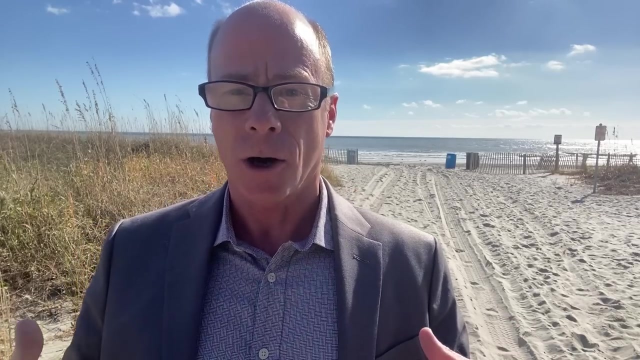 The general public not feeling so good right now. So go ahead, put it in the comments Now. even though they keep telling us the rate of inflation is coming down, it's not the prices that are coming down. Now you have to remember: prices are still going up, but they are going up at a slower pace. 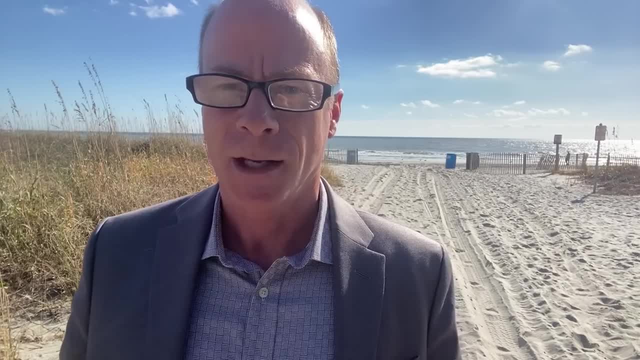 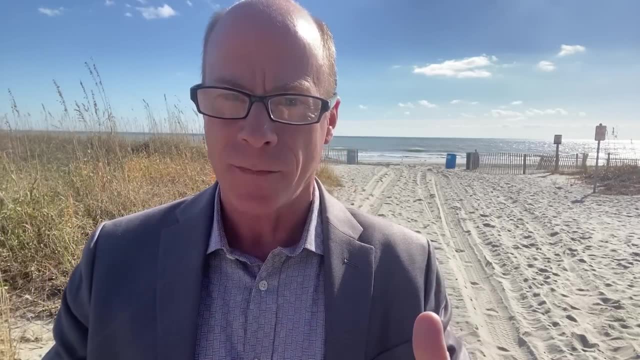 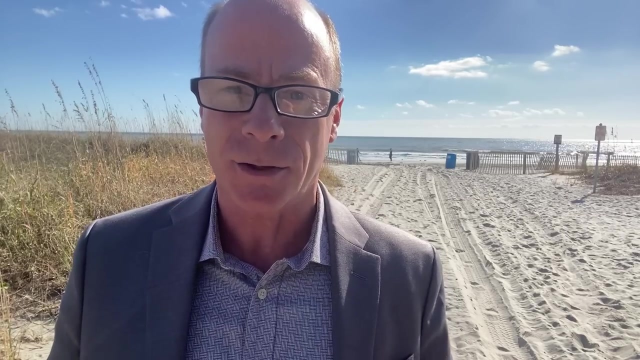 and they're not skyrocketing like they once did. But the truth, it's the compound effect. It's pushing so many And it's affecting all of us, And the fact is, prices have not come down And prices have gone up faster than wages and income. Number five Americans are struggling financially. 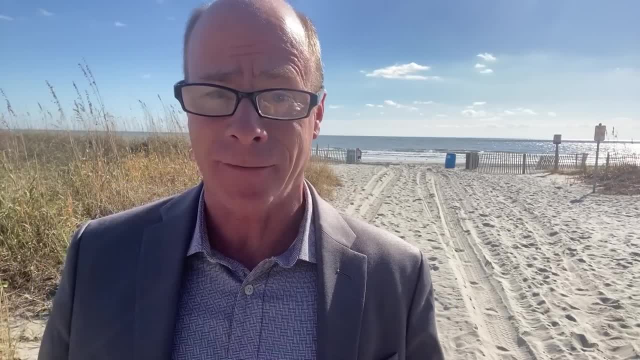 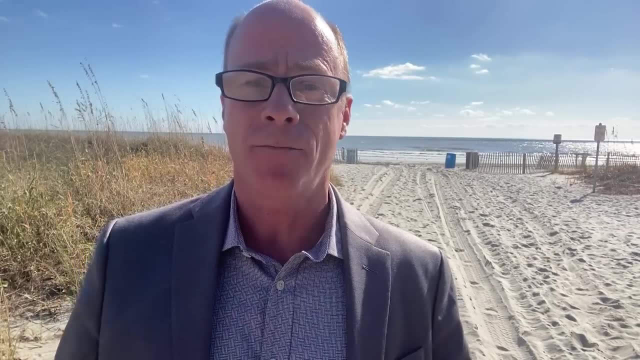 Now, in case you did not know this, the average American is struggling financially, Paycheck to paycheck credit cards, running in the rat race on the treadmill. Now look, the media is misleading the public And there's a lot of people that already know this. But if you put the gap between, 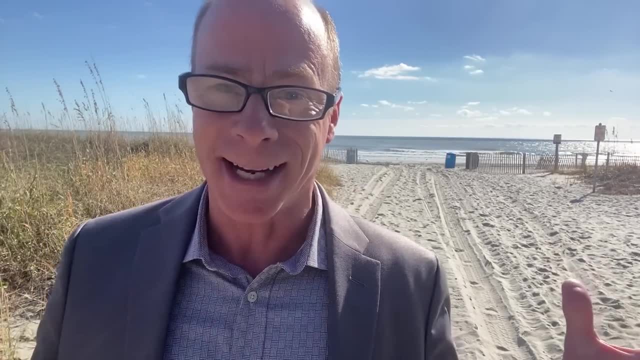 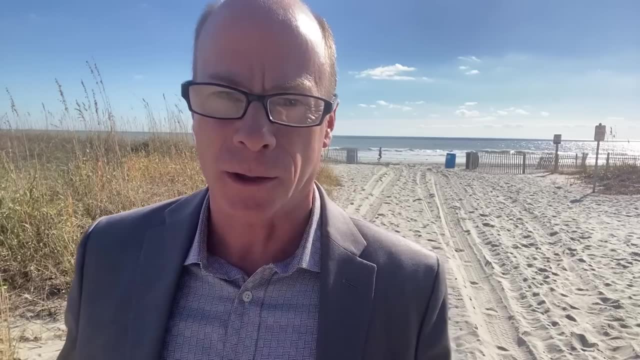 getting ahead and getting further back, you're going to have a lot of people that are going to behind. It's widening, So I'm going to expose this fact Now. just take a look at the same households. Some households are financially strong. They live in the American dream And 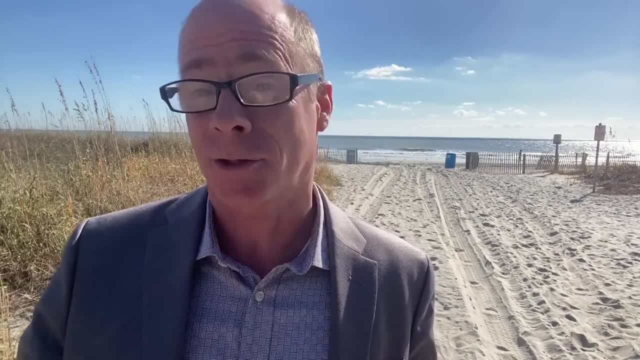 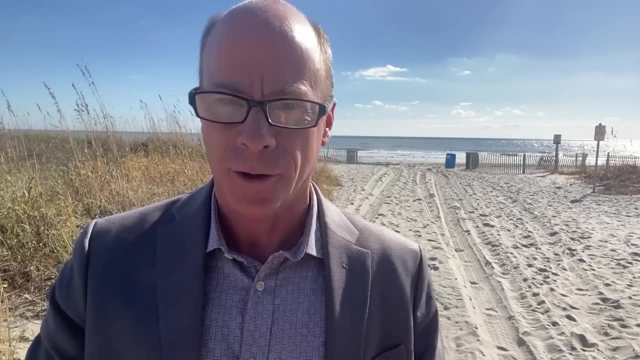 they have the foundation of a home of their own And they're not paying rent to someone else And they're taking advantage of the tax breaks that homeowners receive. Now, on the other hand, there's others that just can't get ahead, And with this continued inflation thing, 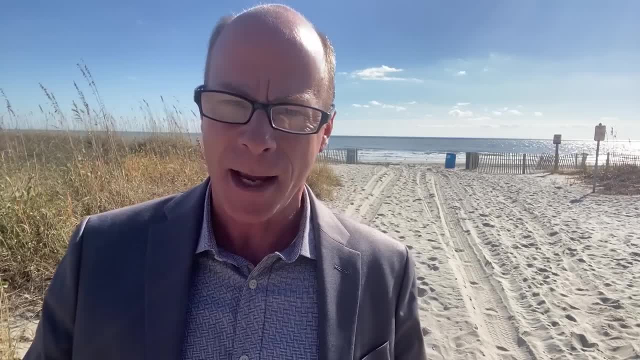 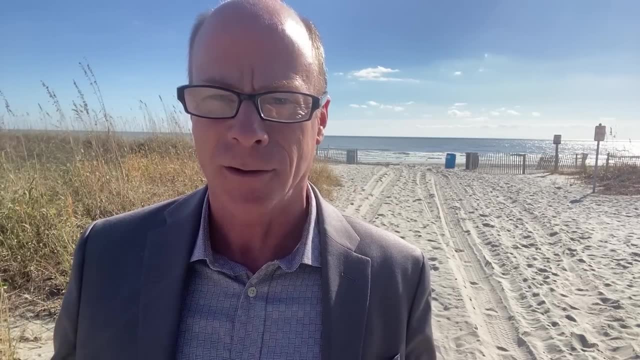 they're literally slipping further behind every single day And the media and the system wants you and I to believe that it's really good to have all these new apartments that are being built. Have you seen them where you live? I mean, let me know, But the media is lying at the rate of 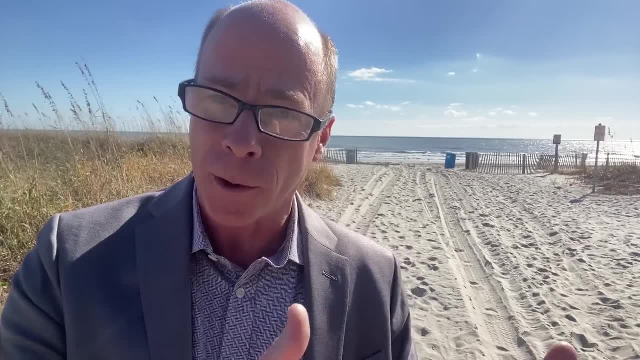 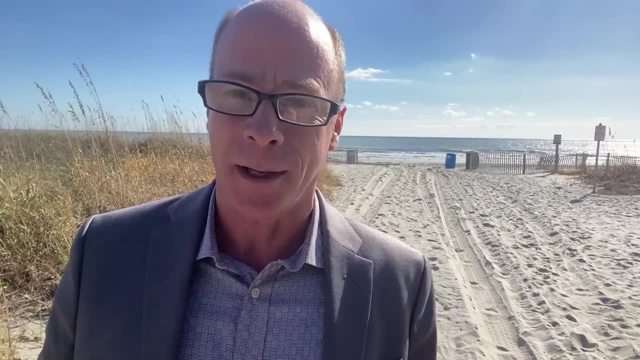 inflation, Because over time you can either work for you if you've invested or it can work against you Now, because if you're renting when you get older, in retirement, you're going to continue to pay those inflated rent prices forever into the future. And also number four: 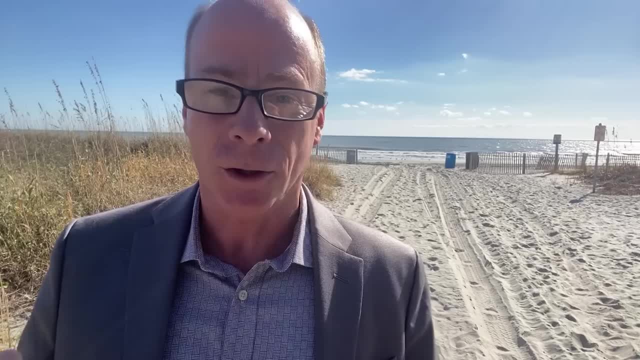 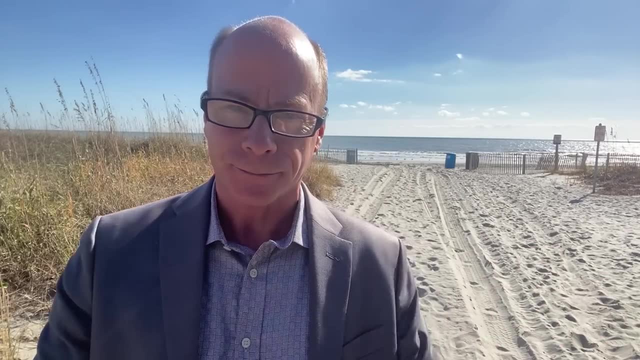 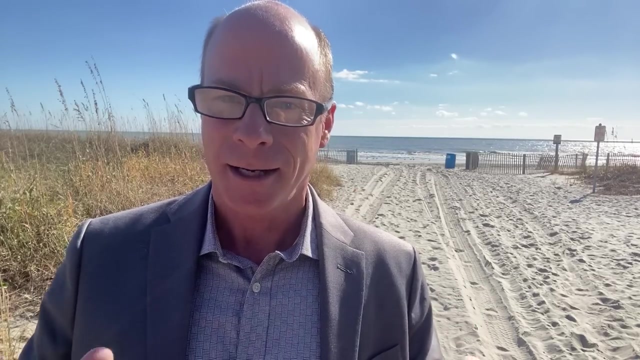 the warning signs. Now the media says the consumer is still strong, But there's a major distortion of the truth And, as I said, I want you to look at those broader economic trends. Let me explain this. Savings are down and will remain down for years. What? Yeah, And here's why. 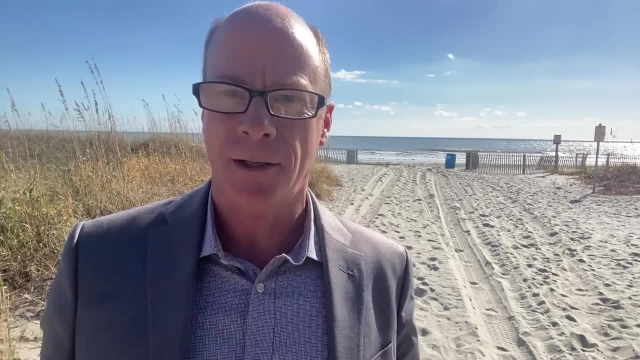 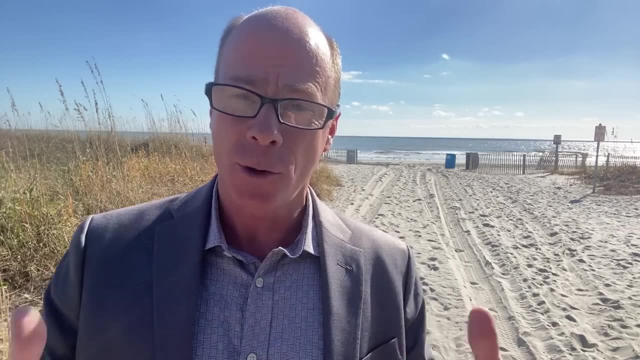 Because many of the baby boomers who retired are now dipping into the savings to pay for their lifestyle And they save for retirement And it's their time Now. they're buying new homes And they're moving to places like where I live, And I've talked about this in many of my previous 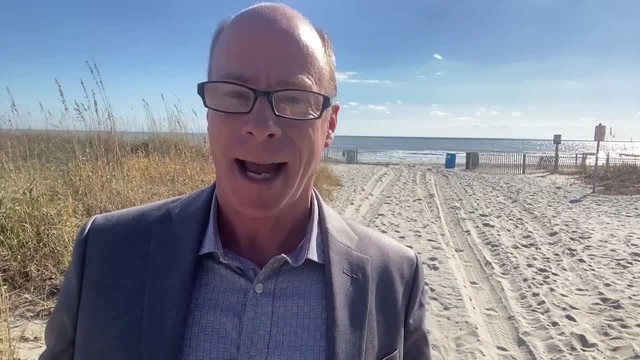 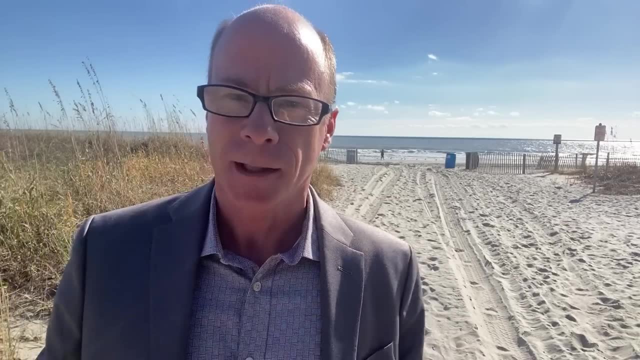 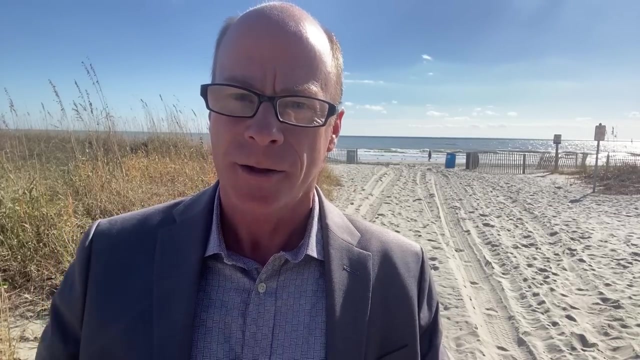 videos. But the truth is spending is actually down even further if you adjust for inflation. Let me show you- It's very important that you have the story straight Now. they show you a report that says consumer spending was up at 1.9%, And those are lies. Because here's the thing, The 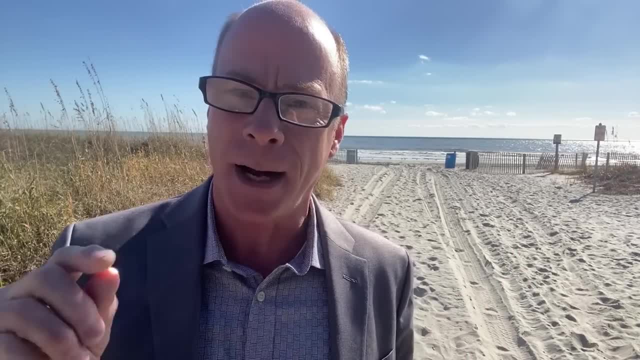 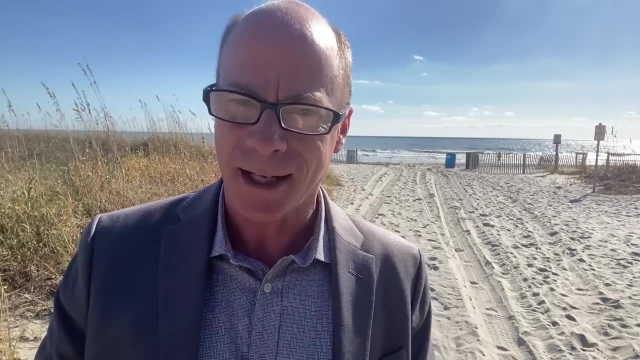 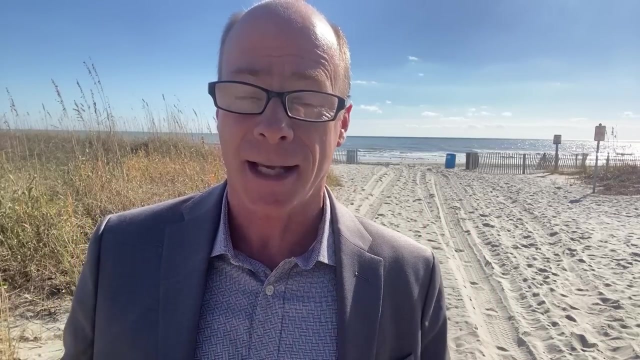 translation of that is: sales were up 1.9%, But with inflation being at 4%, sales were actually 2.1%. Does this make sense to you? Number three: prices will continue to go up. Now, if they ever admit to the truth, that is, things rarely go down in price. Now let me show you this. This is a 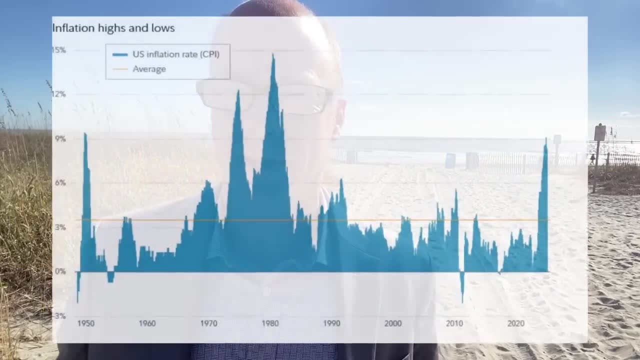 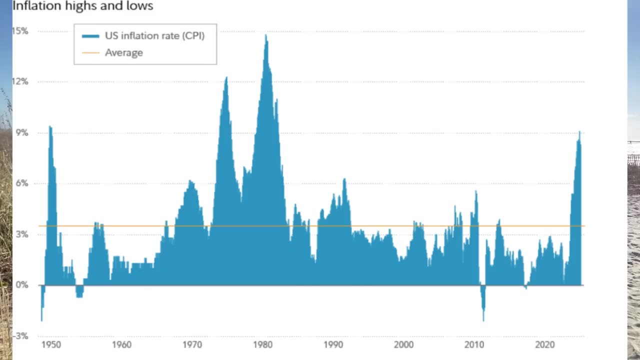 graph. This is inflation every single year since the 1950s. Now look at how much stuff goes up every single year. Only a couple of years it went down. Now if you think about if you bought a house 30 years ago or 20 years ago or 10 years ago, you know. 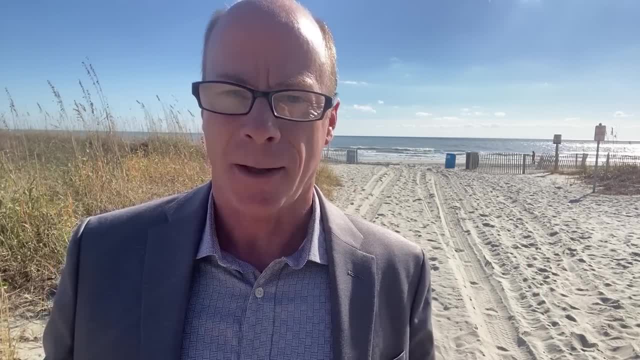 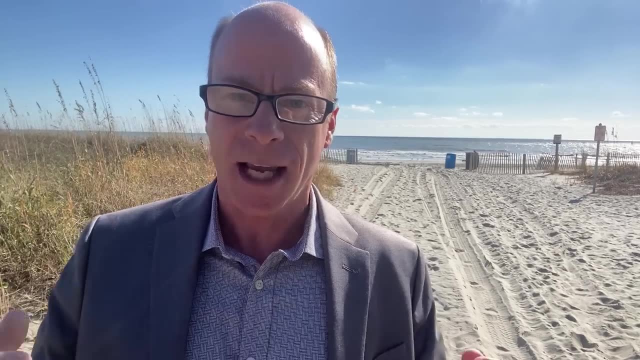 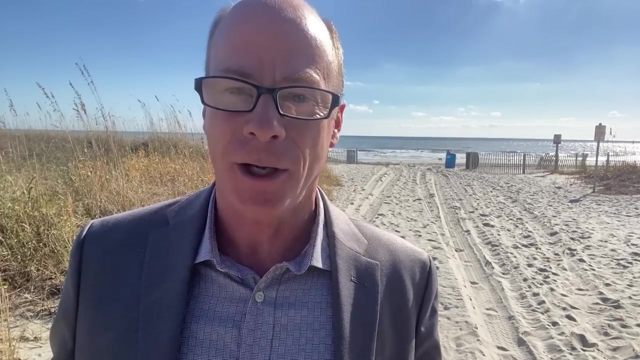 this is why they call it the American dream And this is how the average person can get ahead in life. So the inflation rate we see every single year, this keeps raising the price of buying a home or buying a car or whatever it may be that you buy. Every single year it's going up Now. 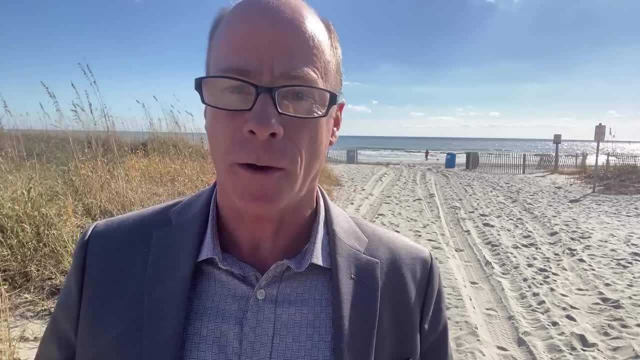 people 10 years, 20 years, 30 years into the future. they're going to look back at this point today and they're going to say- I'm going to let you fill in that blank- What do you think they're? 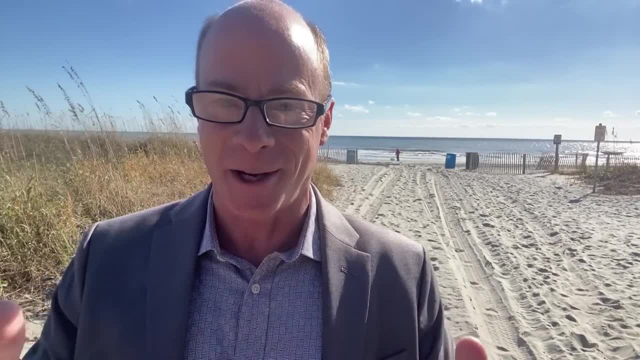 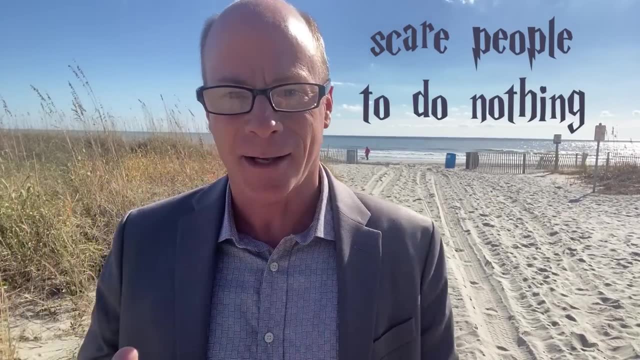 doing So. let me know. I'm looking forward to reading some of your stories. Number two: scare people to do nothing, Now frozen in their tracks. Nowadays, you see it, There's many YouTubers that are using clickbait or crash or bubble or recession just to scare people and get. 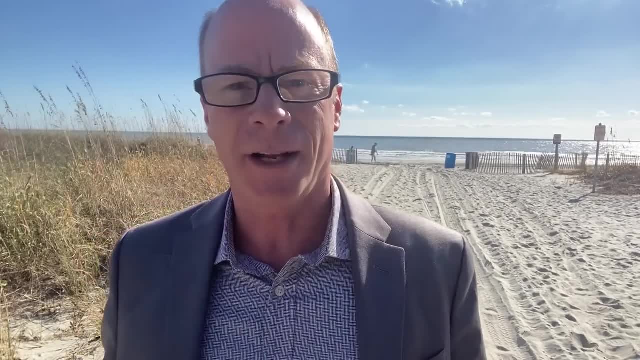 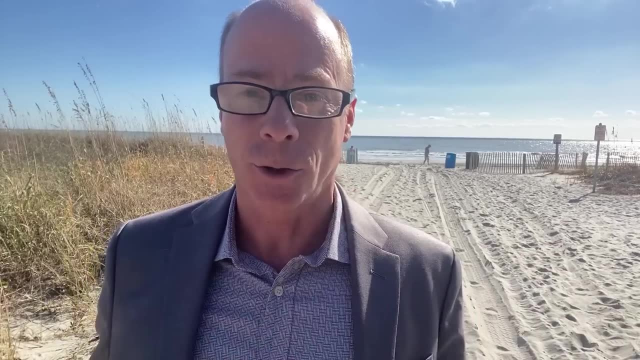 views, which is great for the entertainment part of it, But most of those videos never have a solution. So be sure that you're informed, You know. think about if you had listened to those videos for years. they said that prices were crashing. They said that 50% off deals and they. 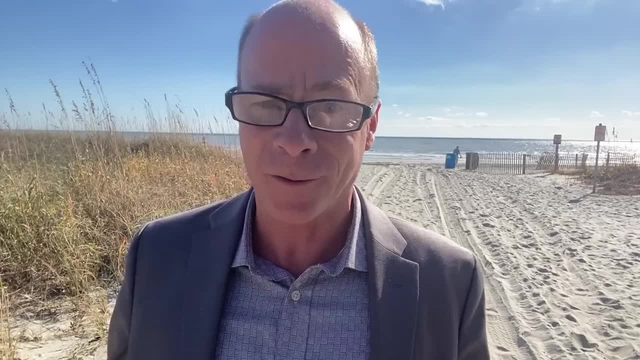 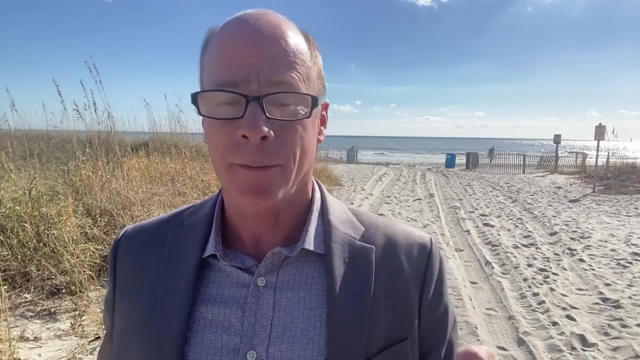 said that foreclosures were everywhere All the while inflation took prices even higher. Now you got to look at the broader economic indicators, as I said. So here's the point: The economy: it's not booming, And at the same time, the sky's not falling either. Looking ahead, here is the 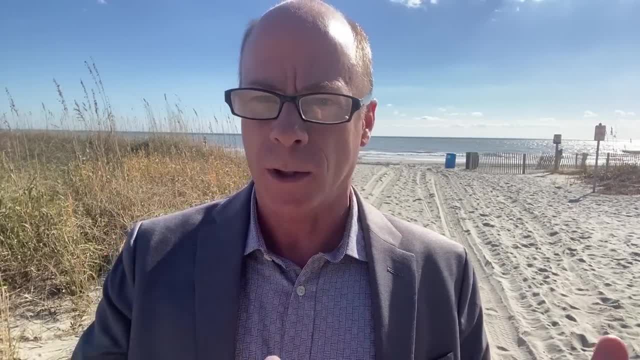 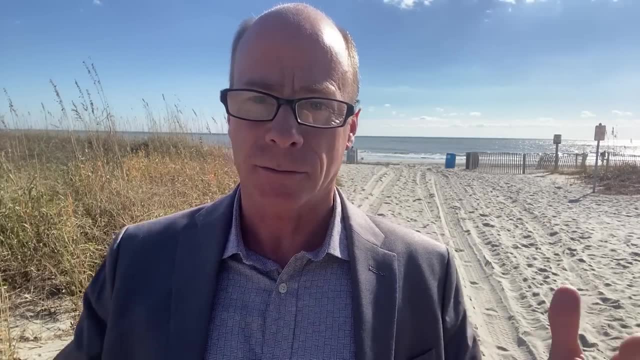 picture Good deals If you know where to look, what to look for, there are still some deals. They happen And, as I've mentioned previous videos, my team has seen some divorce sales or probate sales and where a family member 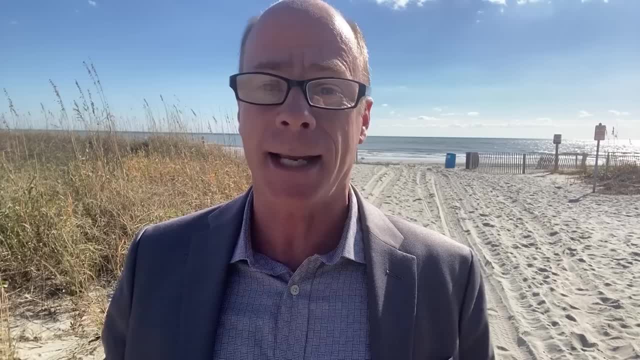 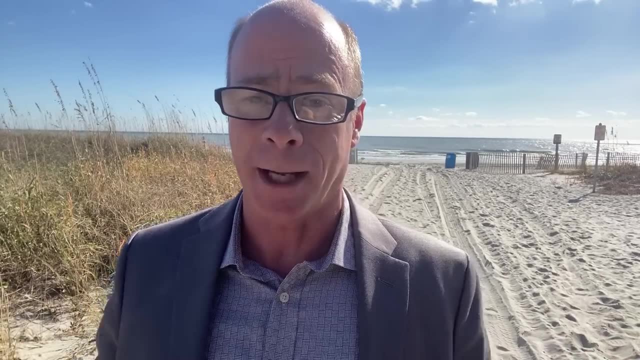 just needs to get rid of that property at any price. But there are many examples of what is a good deal, So that's not the only thing. But just remember, the deal of the decade does happen about once a week, But looking ahead into the future, here's the picture, Affordable. Well, just remember. 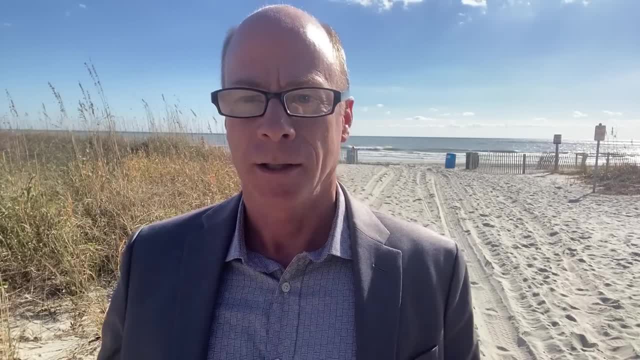 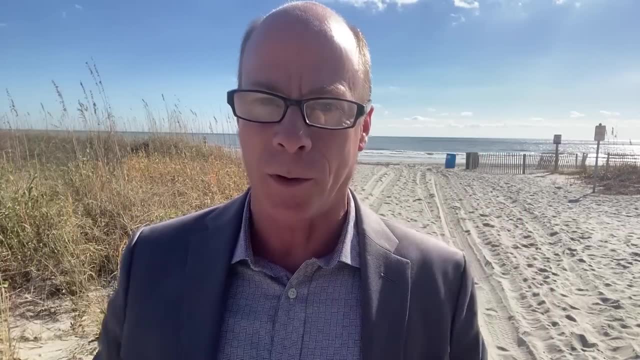 the good is seldom cheap and the cheap is seldom good. Now I have been a real estate investor for the last 36 years And personally I've been a real estate investor for the last 36 years And I've never seen it where real estate was affordable. It's always been just a little. 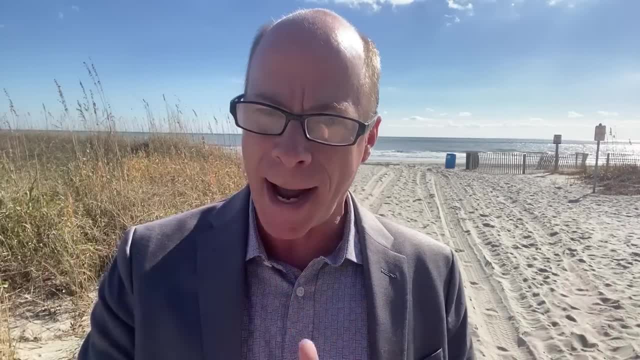 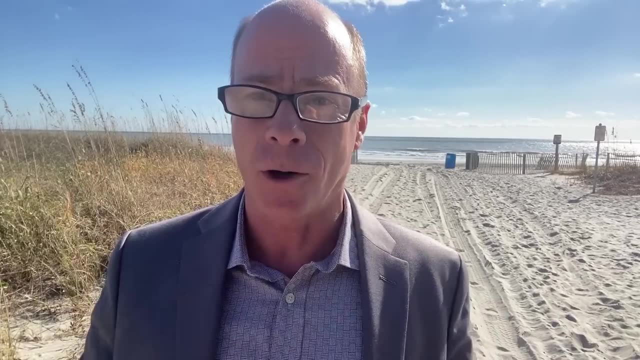 affordable or a little out of reach. But whenever I look back, even the purchases that I made from last year, I'm sure glad that I bought where I bought and when I bought. So if you currently own a home, just how much has your house gone up in the last five years or 10 years, right? 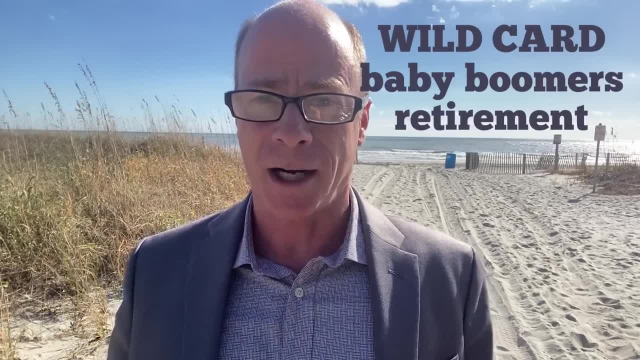 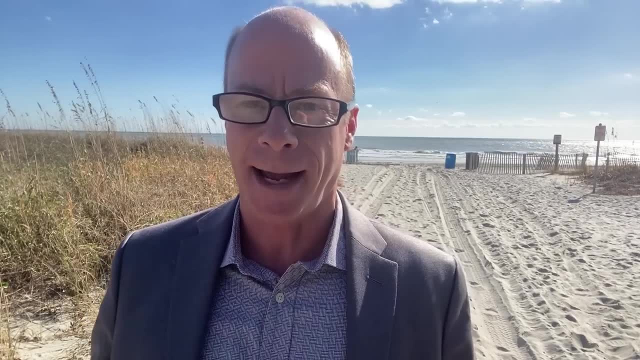 Number one. here's the wild card guys: Baby boomers in retirement. What does that have to do with anything? Well, many of them have worked, They've saved, They've earned whole entire life and they're flush with cash and now retiring all at the same time. Now, 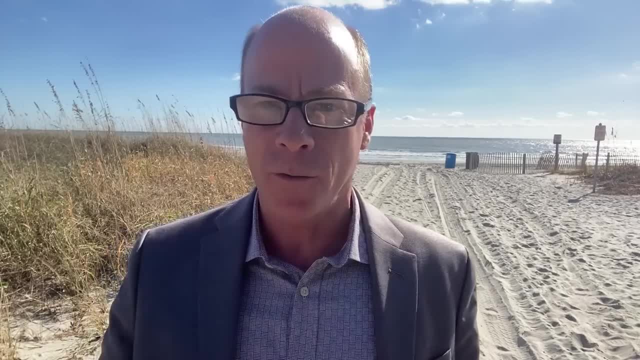 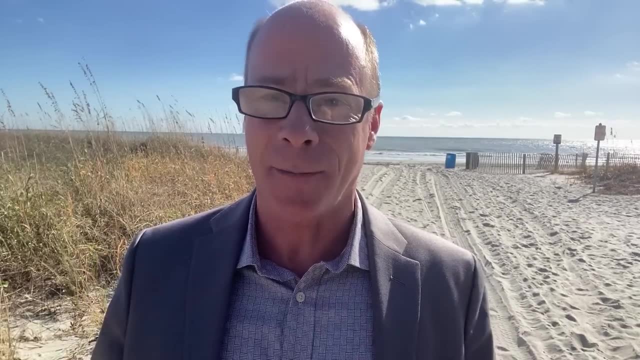 this is a massive population retirement that will all be over the age of 65 by the year 2030.. It's happening And it doesn't matter about the economy. It's nothing stopping this. It's their time. So the question I have for you is this: what's on the cover of every retirement brochure? 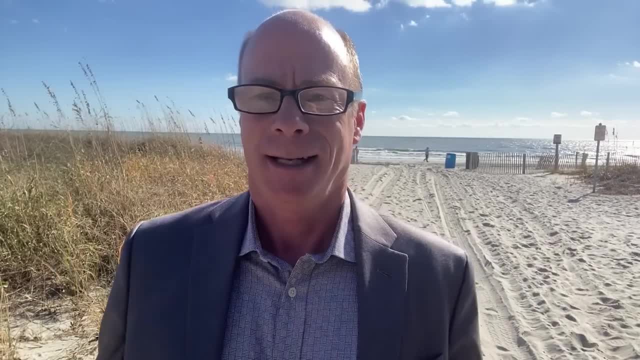 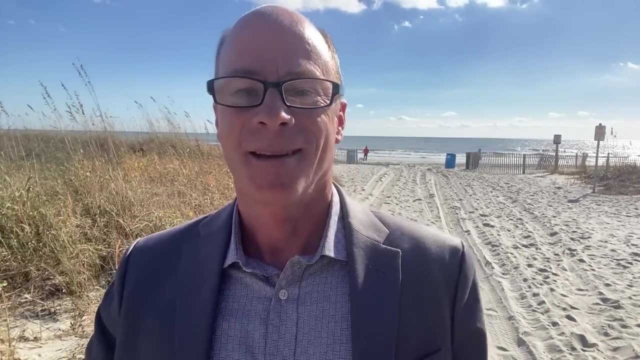 It's this kind of stuff. right, It's the ocean, It's the beach, It's like we've been programmed and the bell goes off. How did I move to Myrtle Beach, South Carolina? Look, many are moving to warmer weather.